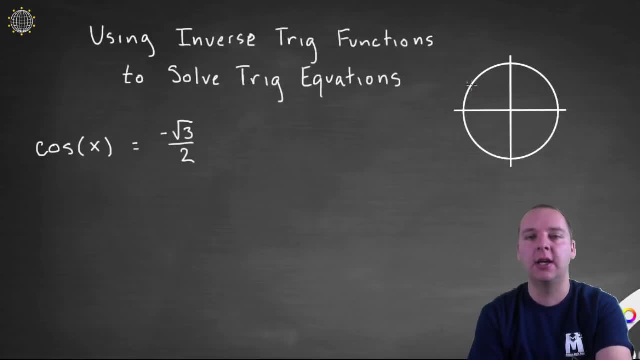 an x coordinate of negative root, 3 over 2.. Since we're looking for the cosine value and it would be right here and right here, which would be 5 pi over 6 or 7 pi over 6, and any multiple, 2 pi multiples of those, if you keep. 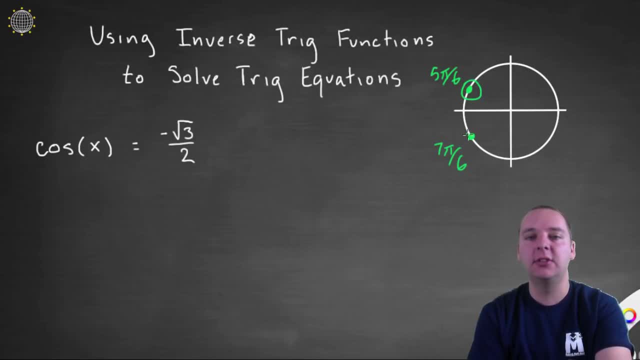 going around and around and around, such that these are your terminal points. So we would get a couple of answers: either x is 5 pi over 6 plus 2 pi over 6.. 2k pi plus any multiple of 2 pi, 2 pi, 4 pi, 6 pi, 8 pi- So we always end up right here- or 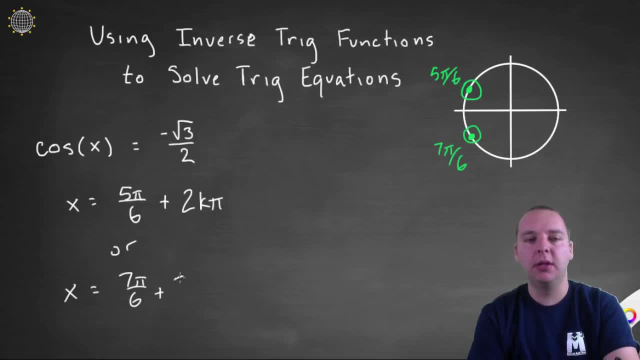 x equals 7 pi over 6 plus 2k pi And, matter of fact, doing it this way even has the added advantage of not restricting our domain. if we we looked at the inverse cosine, you know, if we said our, our definitive answer is x equals cosine, inverse cosine. 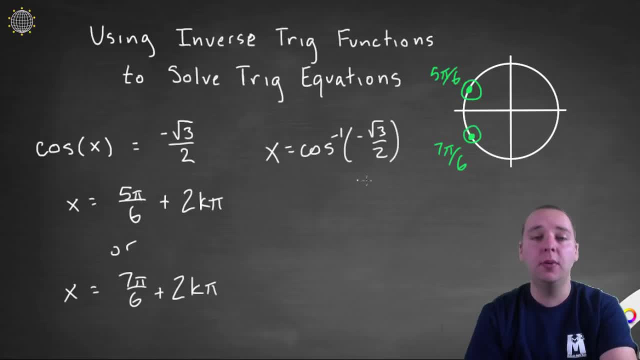 inverse of negative root three over two. You remember this is a one-to-one function, that there's only one answer for this guy. You don't get all the solutions that we should get, like we do this way. So after all that, you're saying: well, Devin, what's the point of this video then? 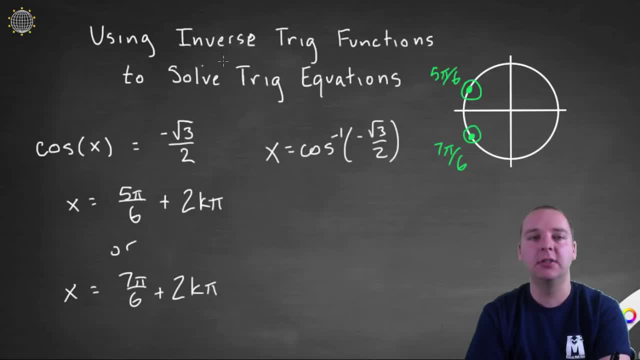 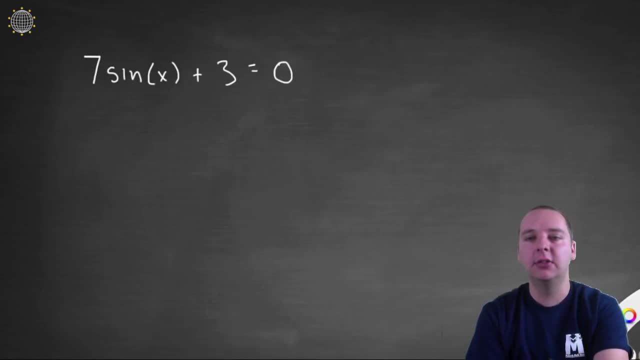 Why are we wanting to talk about using inverse trig functions to solve trig equations? Well, here's why. Let me show you another example and you'll see exactly why this could be extremely, extremely helpful. Let's say we had seven sin x plus three equals zero. Here we go. 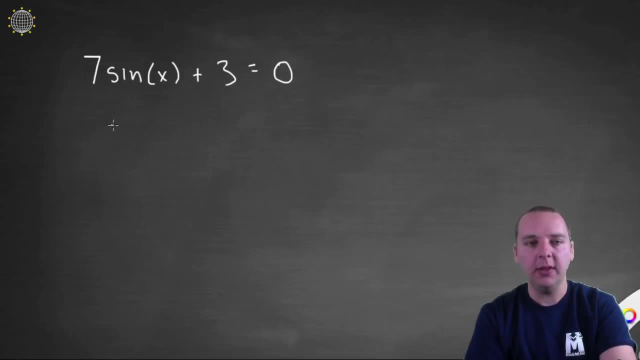 We're going to try solve for x. So we'd have seven sin x equals negative three and we'd have sin of x equals negative three over seven. right Now, on a unit circle, I'm sure that there is a place where the Y and the Y square are equal. So if we have a unit circle, I'm sure that there is a. 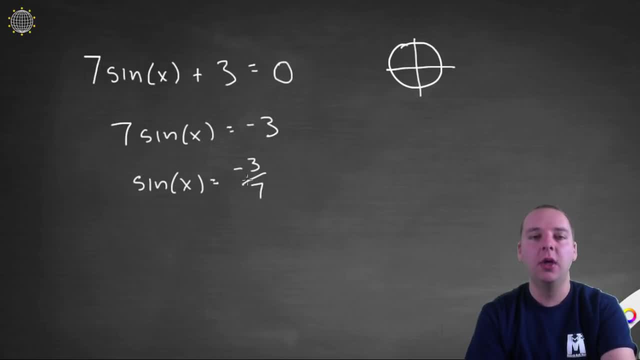 Y and the Y square are equal. So if we have a unit circle, I'm sure that there is a place where the coordinate of the point, the sign of a particular angle, would give you negative three over seven. I could probably even see it as a small negative number. so right about here. so I think those 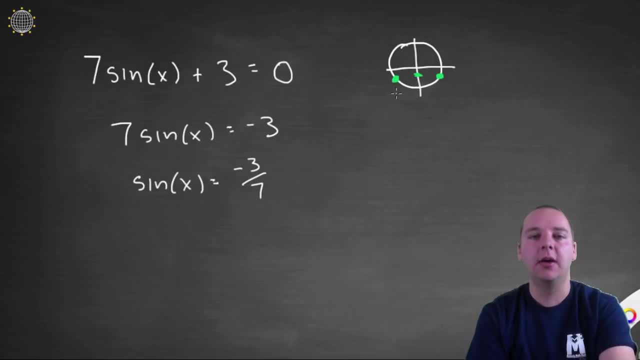 points would be here and here, that would have a y coordinate of negative three over seven. Here's the problem, though. this is not a nice unit circle value. this isn't one of your standard places on the unit circle, so how could we figure out what angle this should be? well, 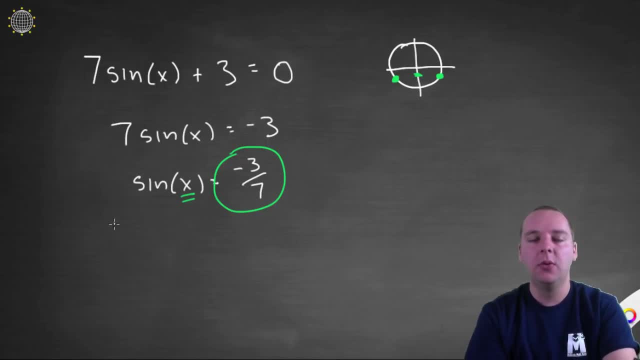 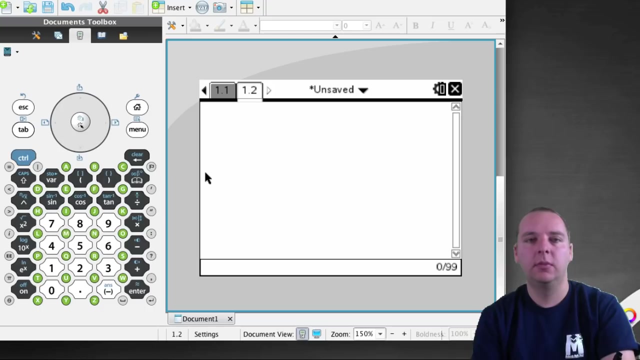 here's where inverse trig functions can be extremely helpful. we can pull out our calculator and we can say that x equals sine inverse of negative three over seven. all right now. so let's pull out our calculator. so here we have our calculator up, and so we need to evaluate. 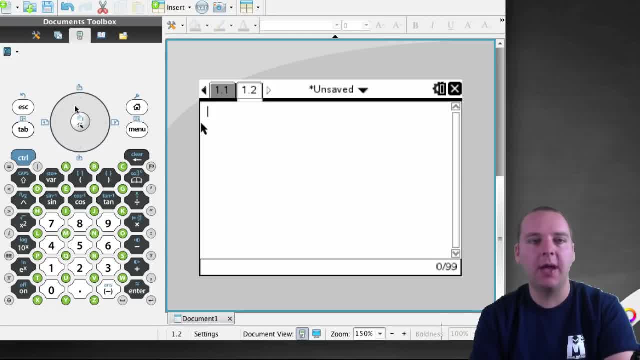 sine inverse of negative three over seven. I'm using a TI inspire, but you can do this on pretty much any calculator. the buttons might be in a different place, But you know, all calculators, at least graphing calculators, have this feature. here's my sine. 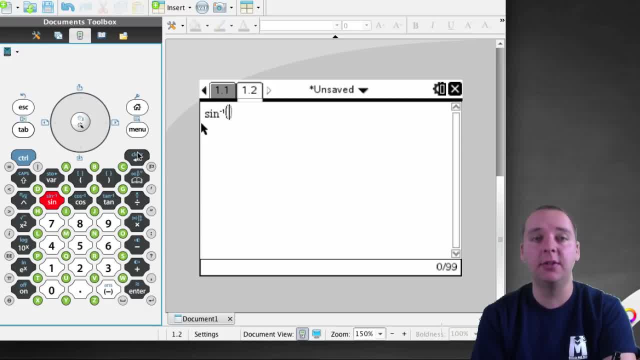 inverse button, so I'll go sine inverse. make sure you do sine inverse and not sine of negative three over seven. now when I push enter, something strange is going to happen. you push enter and it basically looks like it gives you the same expression. it writes it as negative sine. 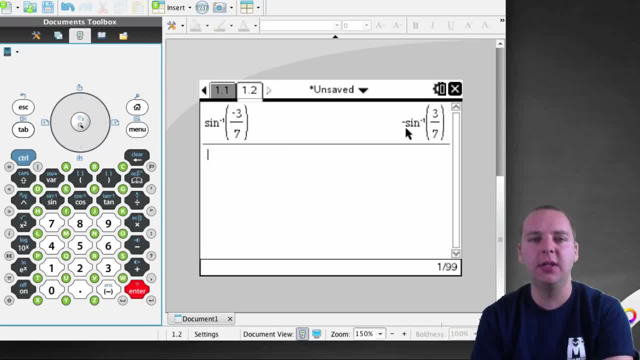 inverse of three over seven. but that's useless. that doesn't do me much more good. What it's doing is leaving the answer as symbolically as it can. it's using some reflective properties and some symmetry properties of the sine inverse graph, but it's trying to leave it in a perfect 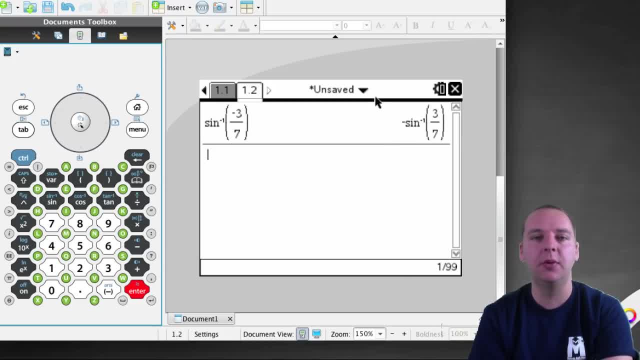 format, not give you a decimal approximation, like we would prefer, and it will be some strange decimal because of the weird value that it is. so here's what we're going to do. I would recommend- This is a little trick to get around- that we'll say sine inverse of negative three point. 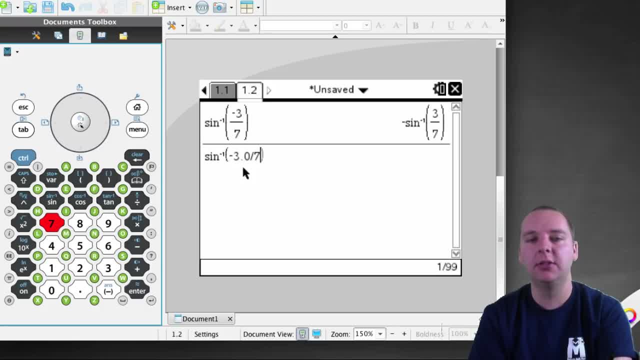 oh, divided by seven. and basically all you're doing here is you're tricking the calculator into, you're forcing it to make a decimal answer, not a symbolic answer, by putting that point. oh, in there, it's the same thing. negative three is the same thing as negative three, point. 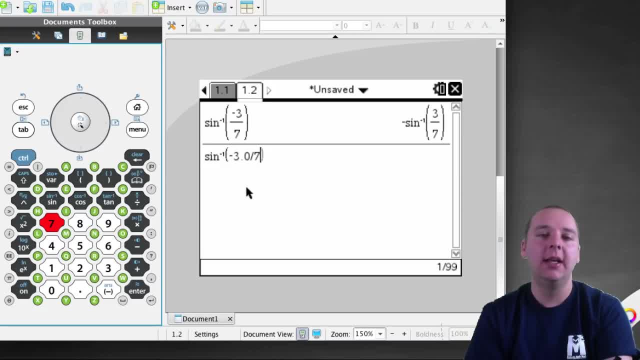 oh, but you're forcing it to give you a decimal answer. Now, that's not the only way to do this. there's ways to convert your exact values to decimals, and what not. this is just a quick little shortcut. ok, so our radian angle? it's not going to be. 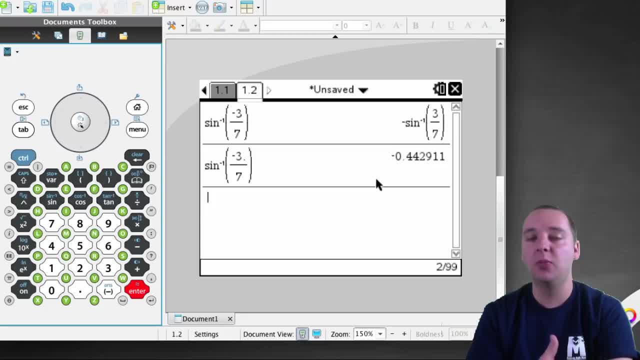 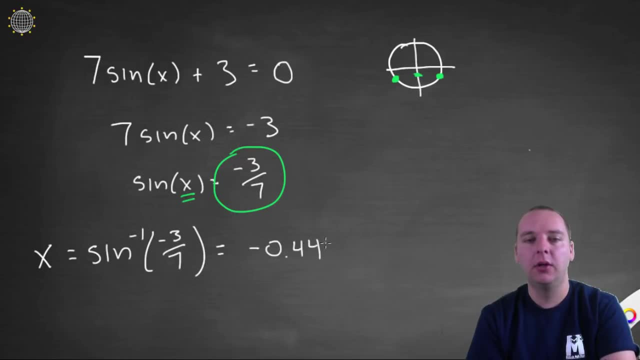 pi over six. it's not going to be pi over two, it's going to be some weird decimal, because our point is not a nice unit circle value, it's negative point four four two, nine. negative point four four two, nine. zero point four four two, nine. now that's this angle here. that's. 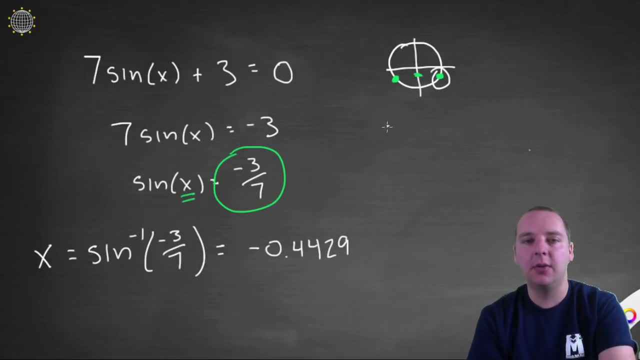 that angle there. So here, let me jot these down- we'll have: x equals negative zero point four, four, two, nine plus two k pi, because remember, you can go around, you know, a full time around the unit circle and wind up here again and again, and again and again. you can add any multiple of: 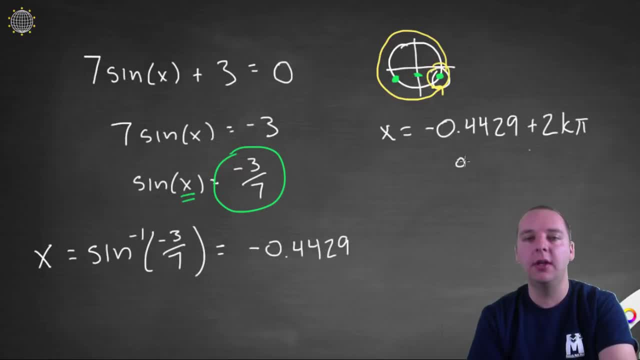 two pi that you want. or there's another angle here- now this one's going to be a little trickier to find- Or x equals. How do we find this guy? because all we know is negative zero, point four, four, two, nine radians below the x axis would be this angle. well, you have to get a little clever here. 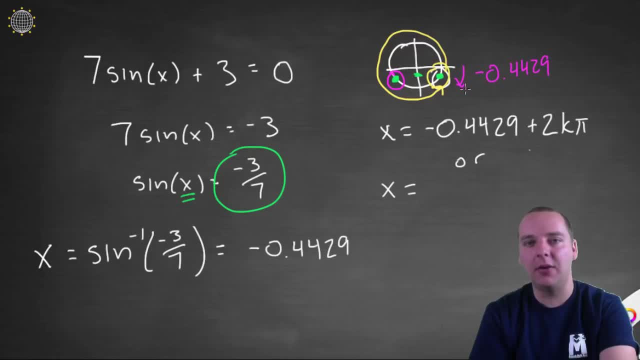 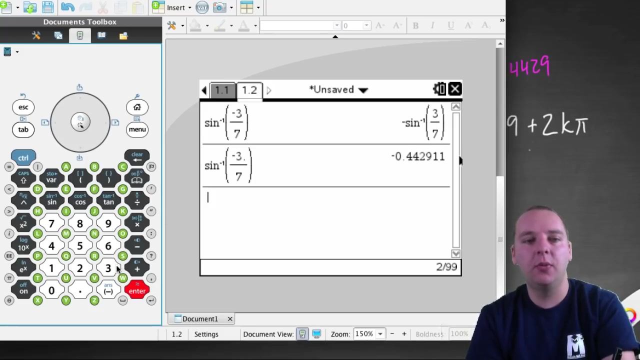 notice. just look at that distance there. look at this angle amount here it's that much beyond the radian angle pi, but in the positive direction, not backwards, but more than pi. So if you realize that you can be a little clever here and we'll go back here and we'll 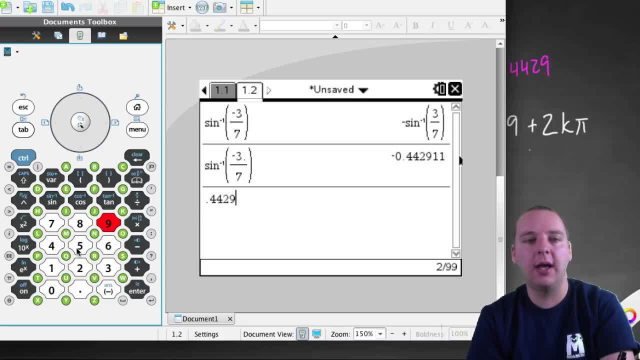 take point four, four, two, nine, one, one, etcetera, the positive amount, because we're going counterclockwise, we're going farther past pi. so we'll take the pi button here and add that radian amount to pi and that'll be three point five, eight, four, five. that's a little larger than pi three. 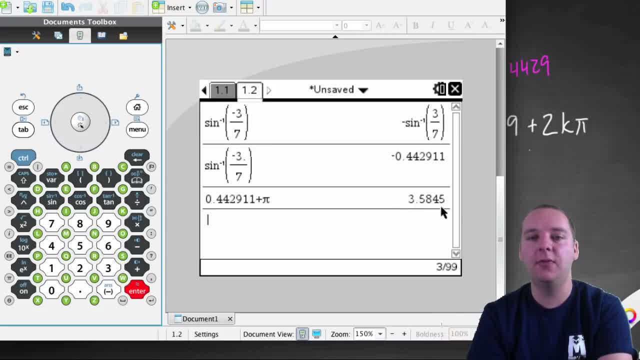 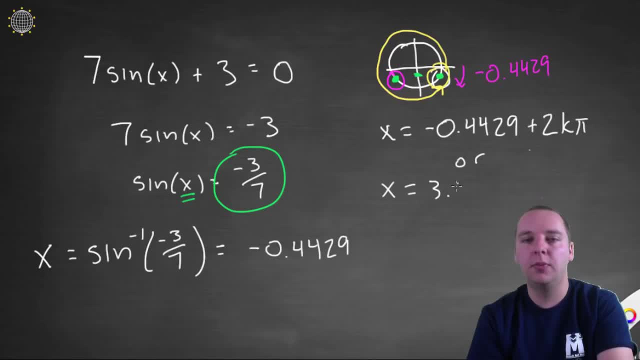 point one, four would be pi. Three point five, eight, four, five. three point five, eight, four, five. same color. three point five, eight, four, five. that's this radian angle, but again, we're allowed any multiple of two pi beyond that. so we'll put plus two k pi. where k is any integer, k could be zero and you get.